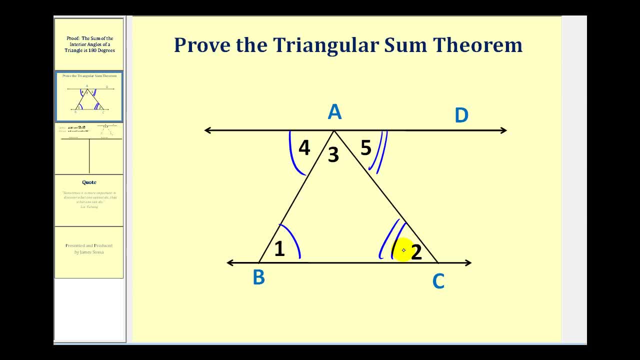 measure of angle five is equal to the measure of angle two. we can perform a substitution to show the sum of the measures of angles one, two and three will be equal to 180 degrees. Now there are a couple other minor details we'll have to address, but that's the main idea behind the proof. So let's go ahead and get. 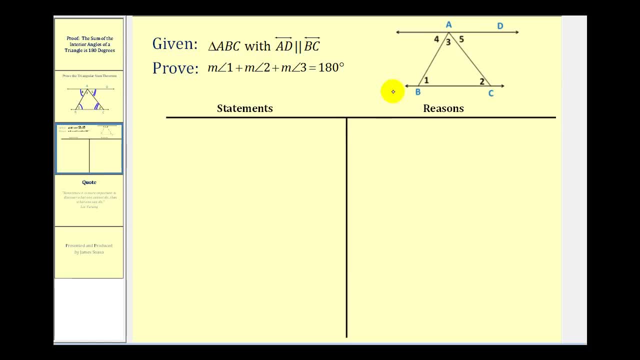 started. So again, here we have the same diagram as on the previous screen, just a little bit smaller. So of course we'll start with a given. We have a triangle ABC with line AD parallel to line BC. Next we'll state: angle four is congruent to angle one and angle five is congruent to angle two. 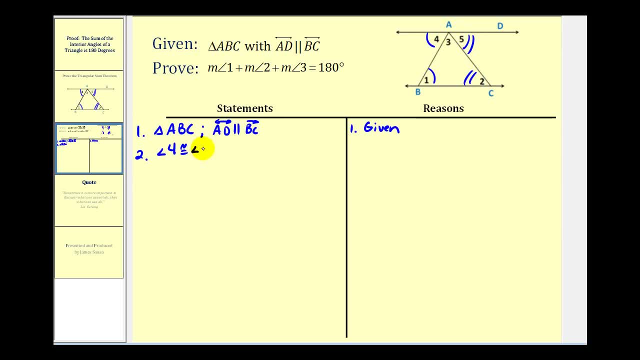 And the reason would be the alternate interior angles theorem. And since these angles are congruent, we know their measures would be equal. So the measure of angle four is equal to the measure of angle one and the measure of angle five is equal to the measure of angle two. This is, by definition of 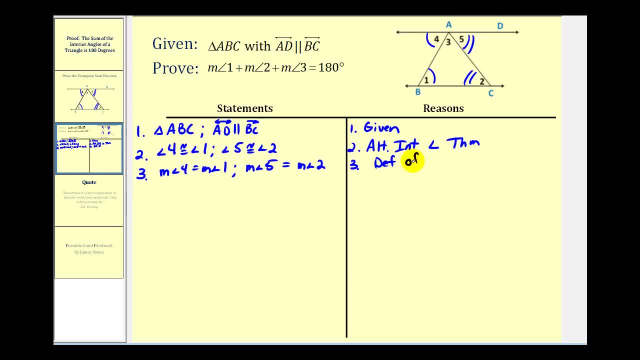 congruent angles. Now, in order to show that the sum of the measure of angles four, three and five is 180 degrees, we're going to have to use the linear pair postulate. So now we're going to say that the measure of angle four 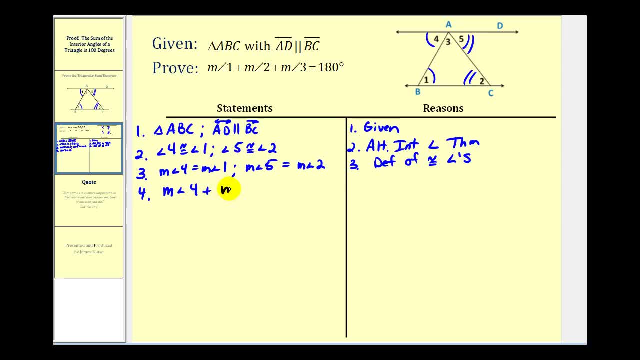 plus the measure of angle BAD. Notice angles three and five form: angle BAD is equal to 180 degrees. Now our ultimate goal is to replace the measure of angle BAD with the measure of angle three plus the measure of angle five, But we'll first have to state that the measure 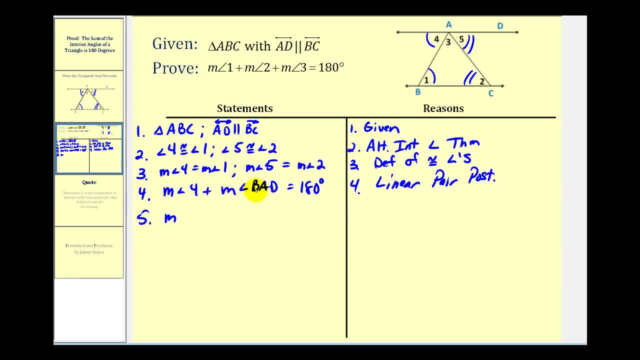 of angle three plus the measure of angle five is equal to the measure of angle BAD, And the reason for this is the angle was 2去了. The next thing is that is the angle addition postulate. Now we can replace the measure of angle BAD.